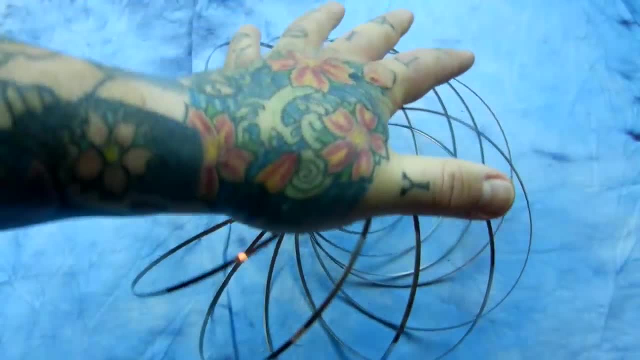 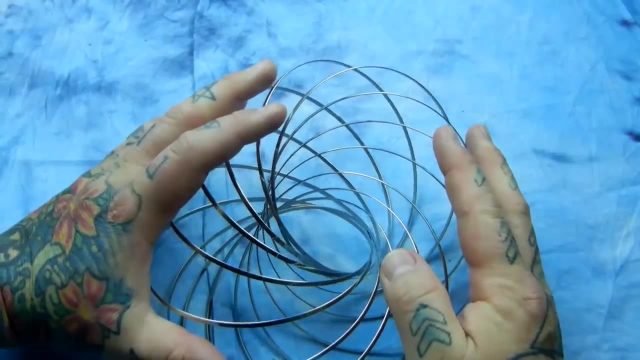 inertia in acceleration. Well, how do you tie all four of them together rationally? Now, actually, let me show you this. Now, as you've seen, underneath the Ferrell cell, a magnet- doesn't matter what shape it is- looks exactly like this. 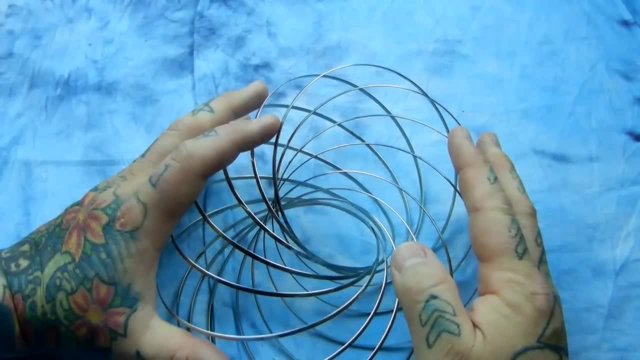 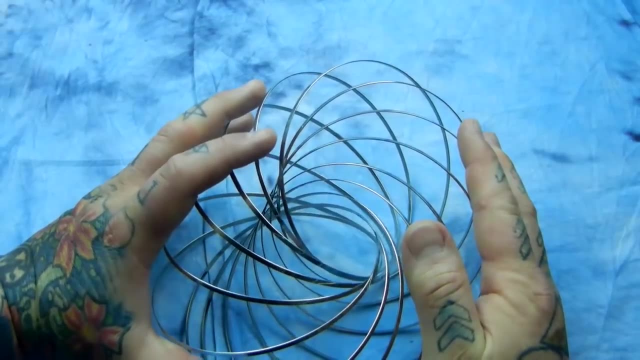 It looks like a torus. It looks like a. well, of course, most people can't visualize that I can: A reciprocating processional hyperboloid which sounds complicated but is divinely simplex. Now you see this spirograph-like. 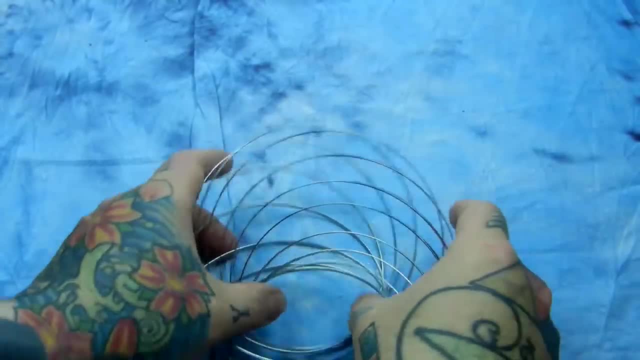 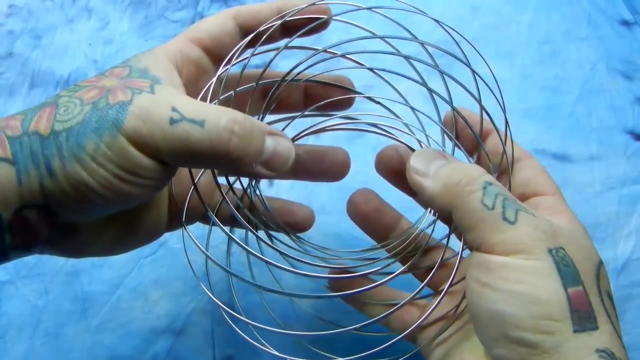 hypertrochoidal pattern. If we're able to get it underneath the camera better, I'll show it to you in a slightly uncompressed fashion. There you go: You actually see a torus, a toroid, a spirograph, a hypertrochoid. That's the expression. 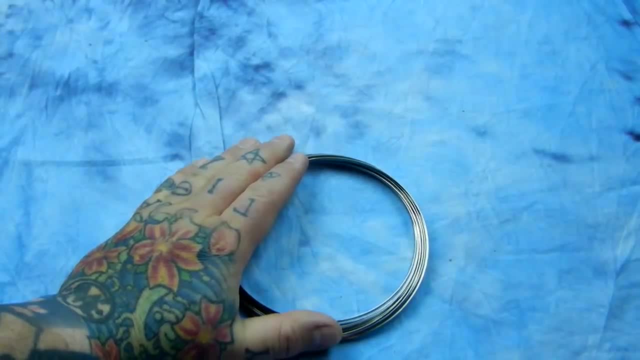 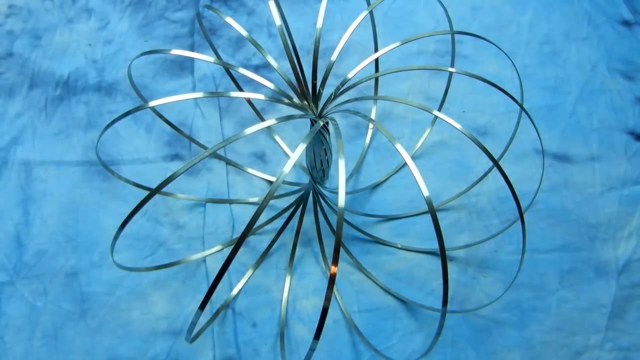 of the loss of inertia. Now, as Faraday called magnetism, he called it the dielectric field. But what does that mean specifically? It means that the necessitated loss of inertia, ie the ether, must be expressed as the creation. 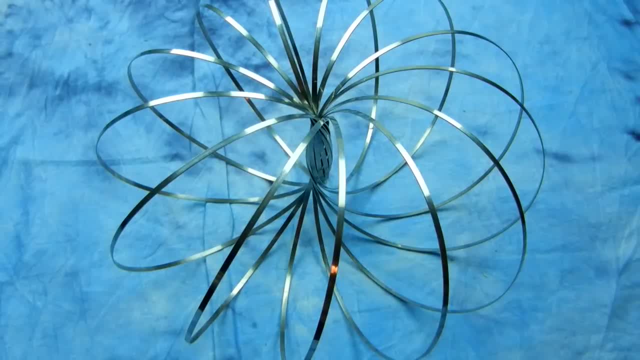 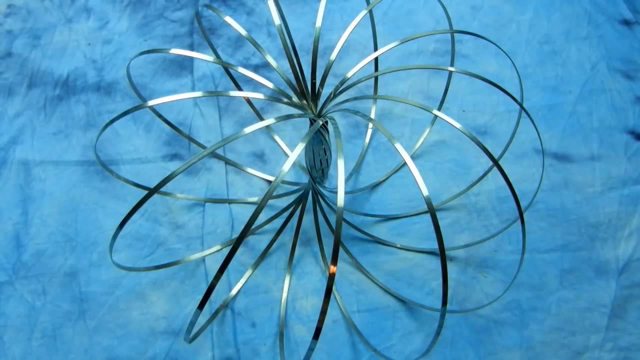 of space and of course the posterior attribute of the creation of space is a measure of movements of magnitude, which we call time. but of course time does not exist. Time is a human contrivance. Here we have dielectricity with absolutely no manifestation. 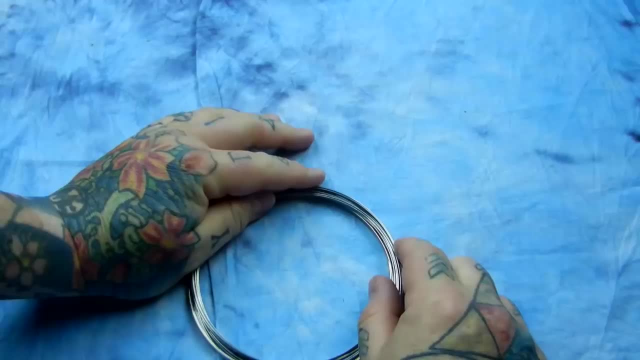 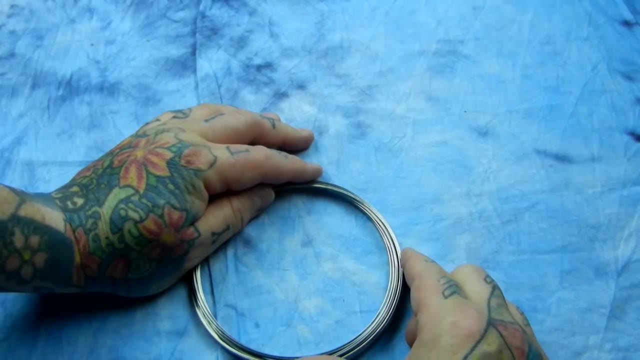 as a linear propagation. Now we think of a single point, ie the ether, as being unmanifest. A longitudinal propagation, such as found in electromagnetism, ie, radio or regular light, obviously has a longitudinal pulse between each. 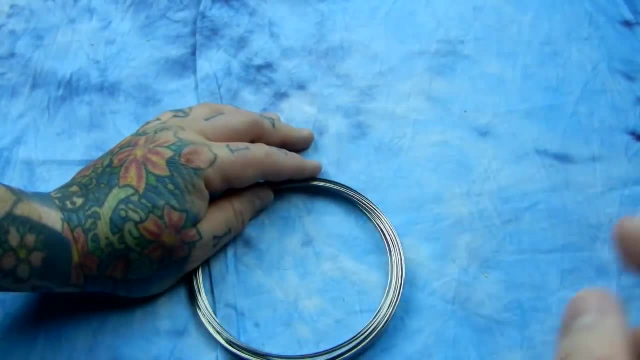 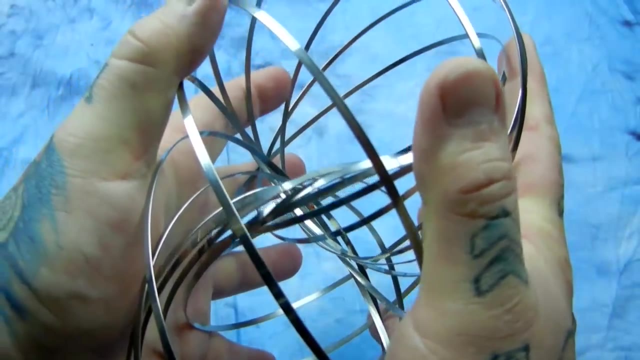 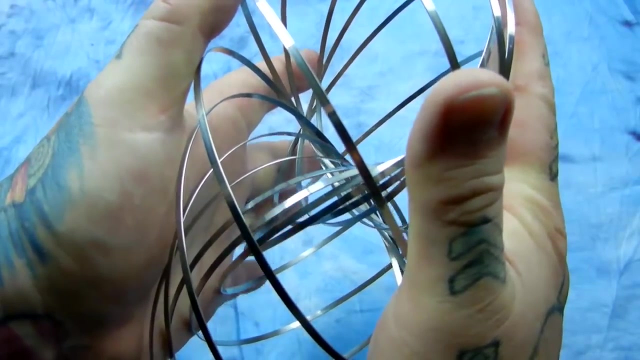 waveform of the electrical value and the magnetic value of the waveform of the transverse electromagnetism. Now here we have electricity, which, by the way, is phi, times, psiq and Planck electrification. Electricity is nothing other than the hybrid of electricity and magnetism operating together. 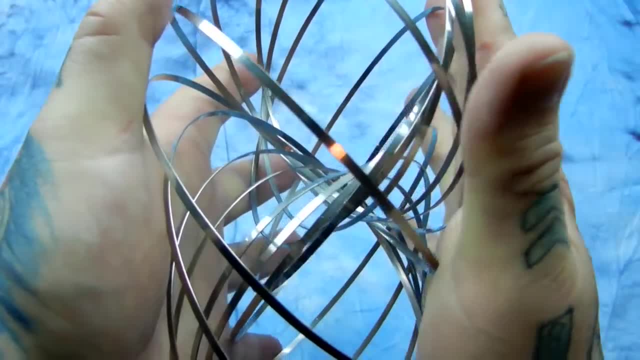 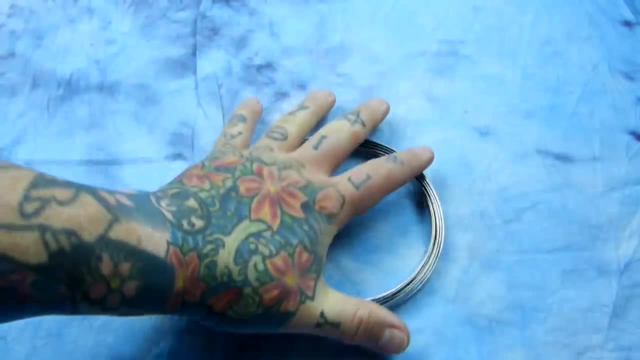 which is found in, obviously, frequency and amplitude, Constantly pulsing back and forth like this: Well, what frequency, What amplitude? Obviously, we have the entire EM spectrum and we have electricity. So electricity is a hybrid of dielectricity. 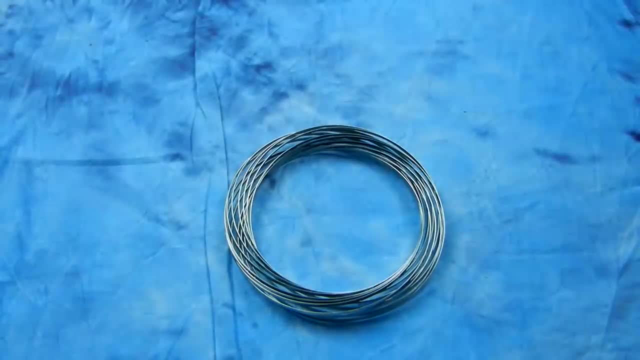 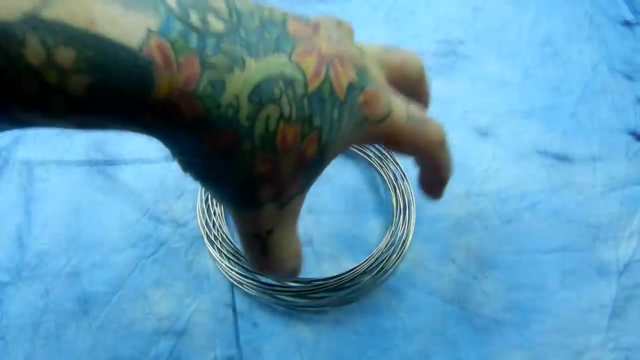 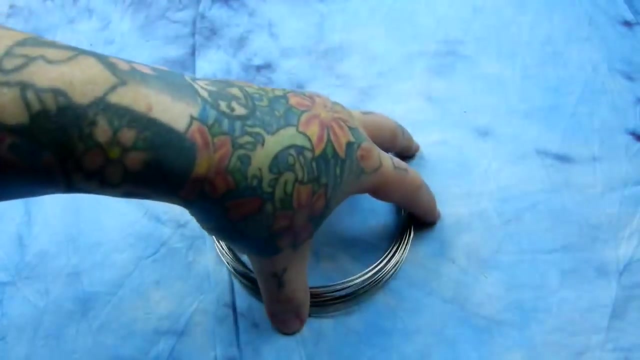 and of magnetism operating at a frequency and an amplitude Obviously so. Now, in the case of- and to make this really simple so that a child could understand- like an electromagnet that pulls up cars, obviously an enormous amount of voltage is actually dropped to. 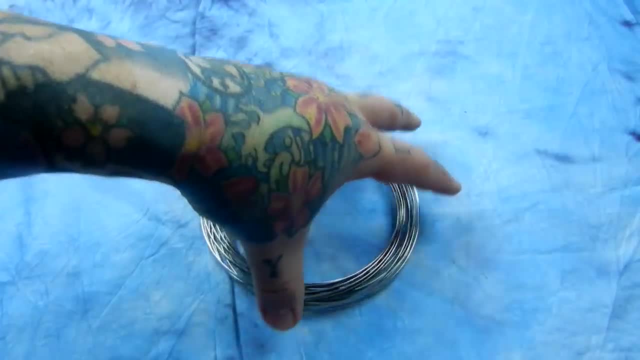 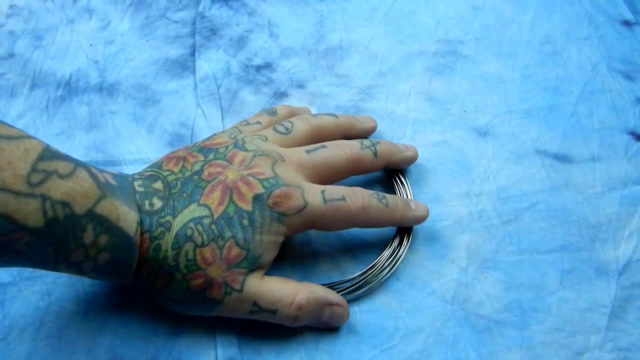 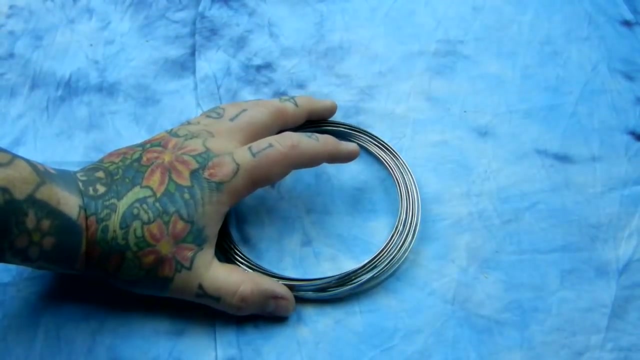 the lifter, like the lifter magnet that picks up dead cars and rescraps out things. Now, electricity doesn't terminate as magnetism or doesn't terminate into magnetism. by dumping that charge and creating a large electromagnet, It loses its dielectric component. So electricity 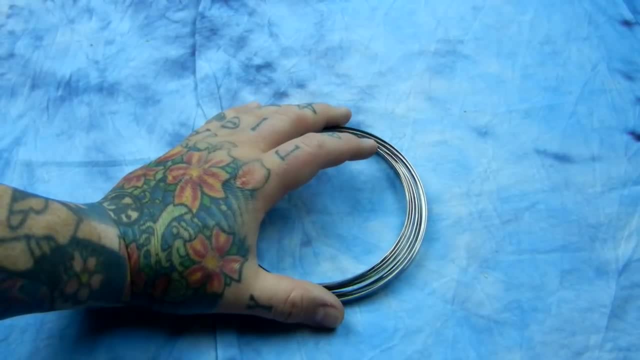 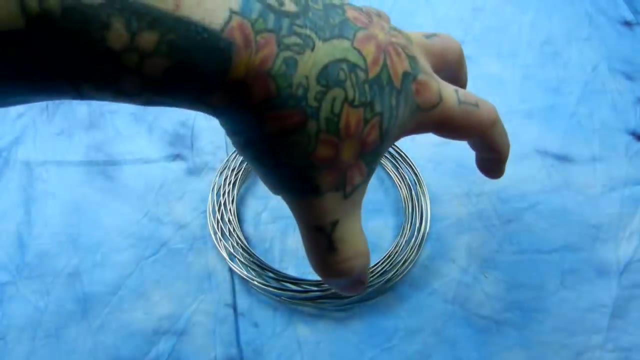 terminates not into magnetism, as wrongly thought, but as magnetism, by losing its dielectric component. In other words, all that electricity that is actually brought through electromagnet to lift up dead cars so they can be scrapped is nothing other than the loss. 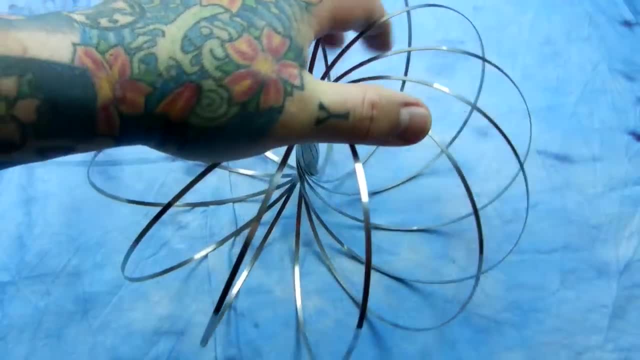 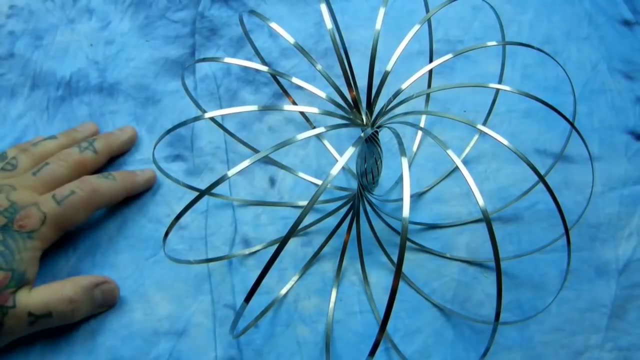 of the dielectric component of electricity, which means you have an extremely high Gauss field that is able to pick up multi ton cars with that electromagnet. It is that electricity terminates as magnetism by losing its dielectric component, not into magnetism. 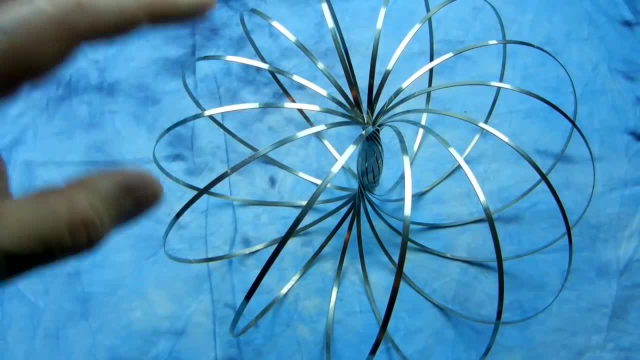 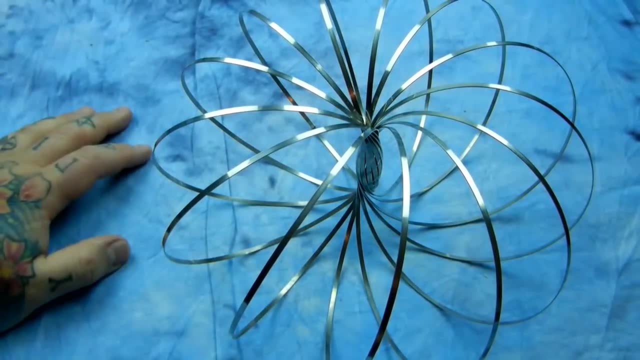 but as magnetism, because electricity is the hybrid of dielectricity and magnetism. Phi times psi equals cube Planck and electrification. Electricity, by definition, denotatively, is a combination of two things: dielectricity and magnetism. So by losing its dielectric, 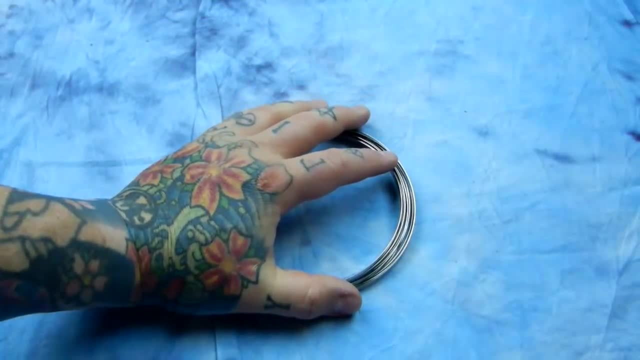 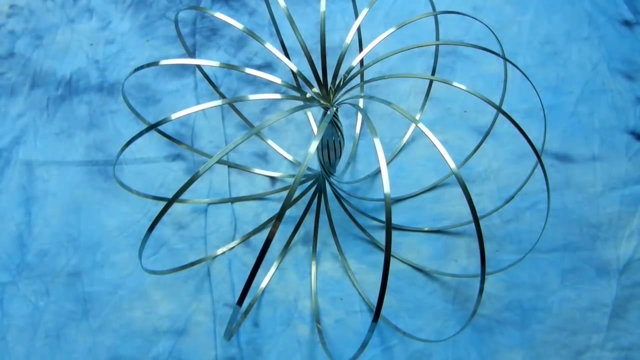 component, the electricity, manifests itself in the electromagnet, for example, as a huge, enormous, very powerful high Gauss magnetic field. Now where does gravity come into play? Well, we think gravity is something different. Now we know, in galactic jets we see enormous amounts of shooting matter. 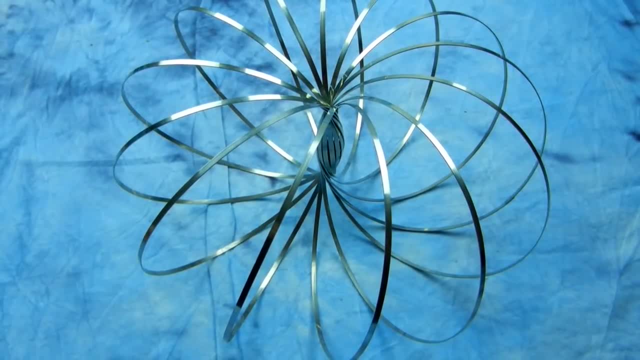 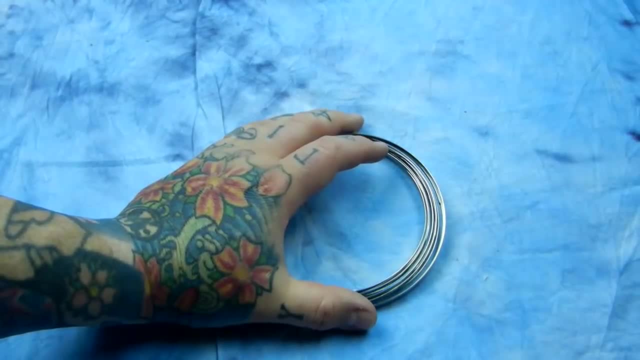 shooting out billions of light years out of either end of galactic jets. Now, the necessary loss of inertia, which manifests itself as longitudinal dielectricity, is an equation. It's 1 over 5 to the power of negative phi, which some people would think would be a number, but it's actually an expression. 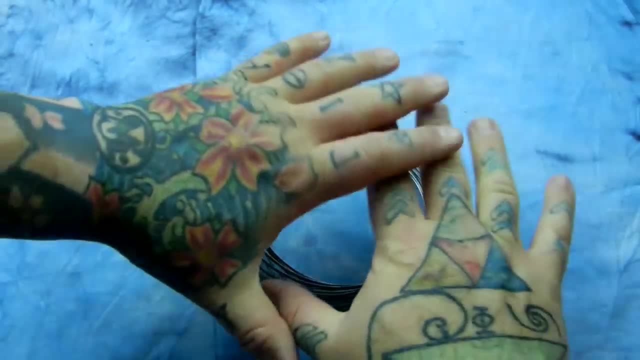 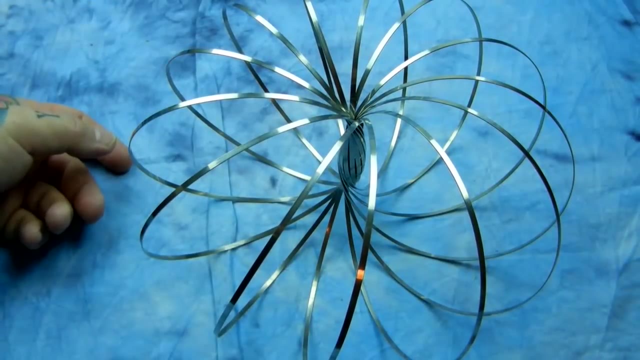 That expression, if we were to think of this as a zero point which is invisible, rather than seeing the circle that equation necessitates the expression which we know, that the attributional nature of the ether expresses itself as longitudinal dielectricity by that equation. 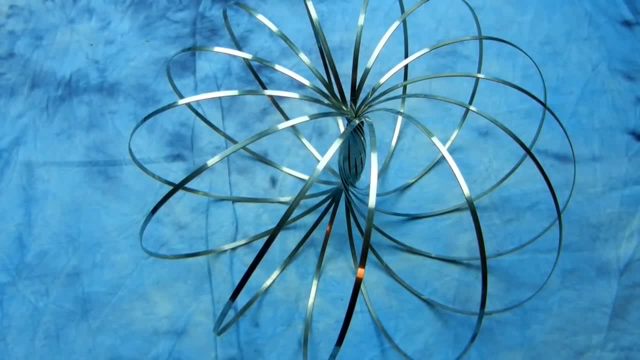 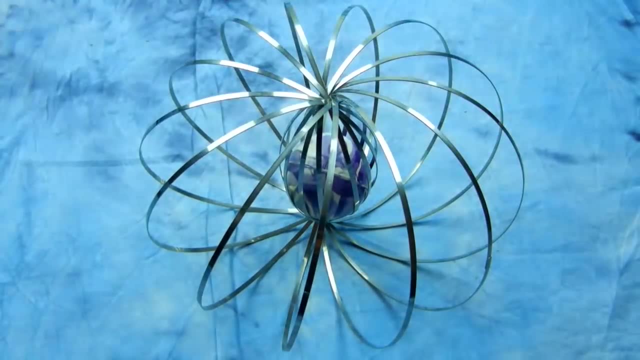 that I discovered 12 years ago. So where does gravity come into play? Gravity, like electricity, is nothing other than a hybrid. So what is gravity? We talk about? what denotes gravity? We're talking about mass. ie matter. Matter is nothing more. 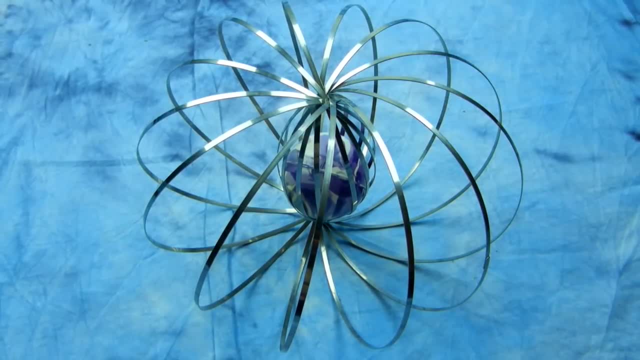 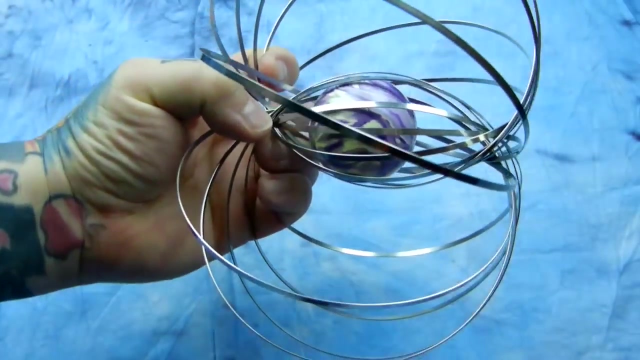 than a dielectric condensate. It's like taking carbon dioxide and freezing it to its solid state. Now, obviously, that is a huge hyperbole and that's a supreme oversimplification, but this is matter Obviously extremely simplex. Let's just think of this. 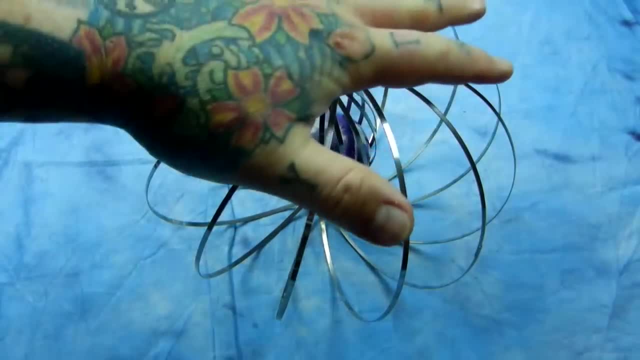 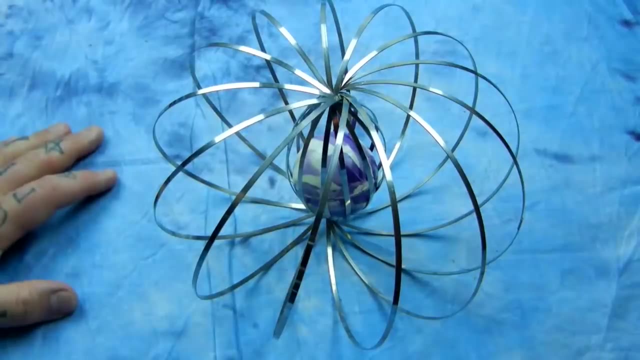 as the hydrogen atom. Even that is too simple, obviously, this model, of course. But we have, as of course modern science likes to say, well, 99.99999% of an atom is empty space. That's not true, This supposed empty space in here in an atom. 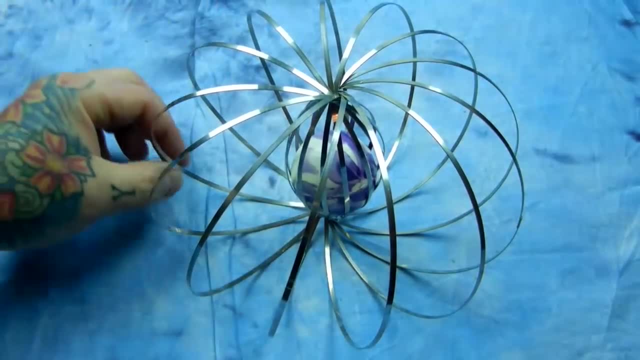 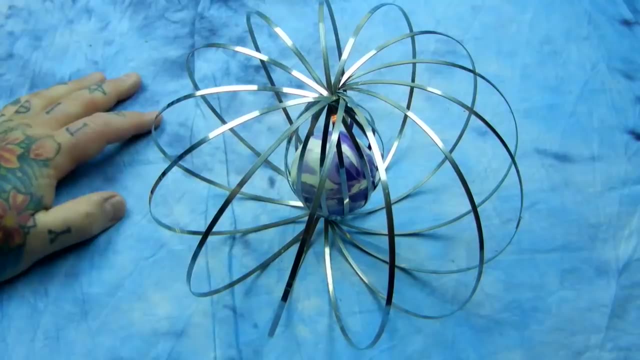 is magnetodielectricity And what we think are electron atoms. Now, by the way, Tesla, Heaviside, Steinmetz, Faraday, even the discoverer JJ Thompson of the quote-unquote electron, denied for a long time. 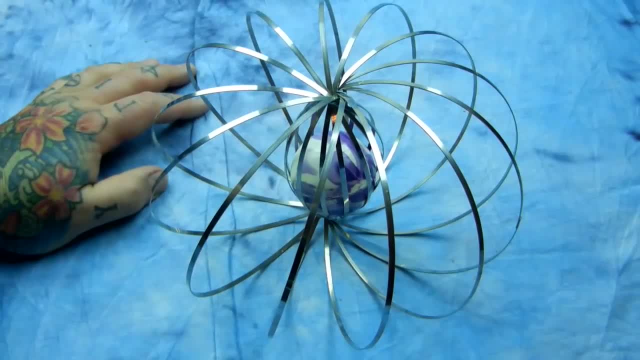 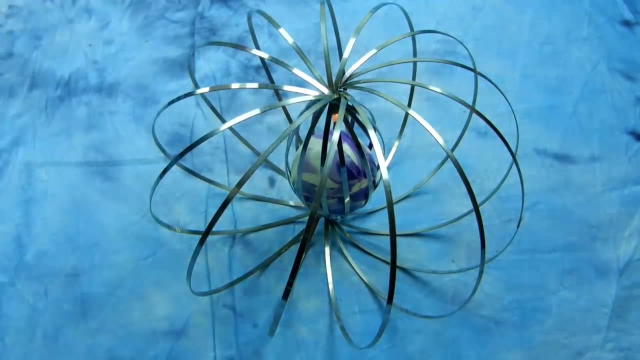 that the electron is a particle. There's absolutely no such thing as an electron particle- And email me if you want a huge list of logical reasoning behind this- But the premise that we have that wires are like huge rain sticks, that little electron atoms are pouring. 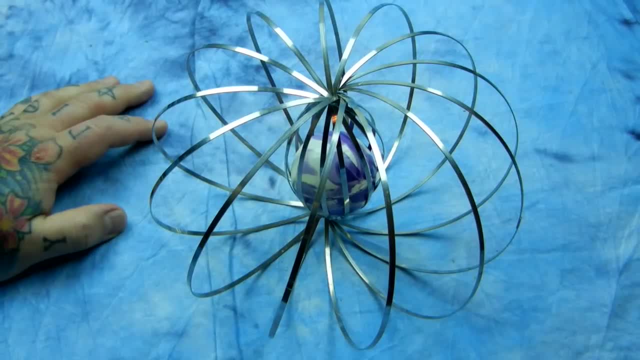 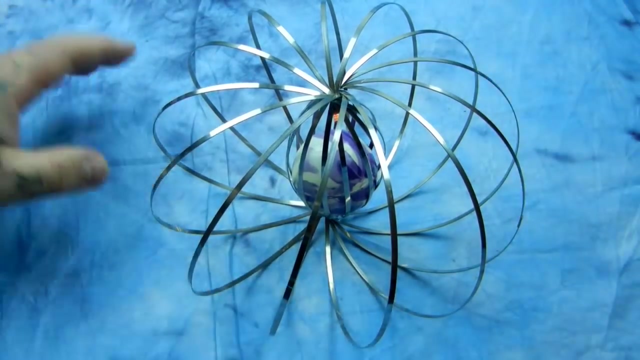 through. Oliver Heaviside called this. I think he called it a mind virus. Eric Dollard called it the same thing. Tesla, on two different occasions, said that the notion that the electron was a particle was absolutely absurd. So everybody that gave you 100% of our current electrical grid, these people. 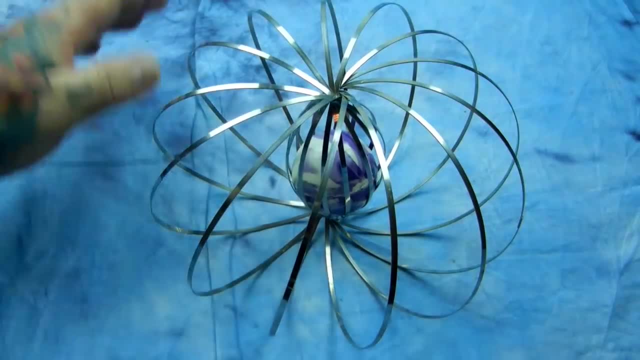 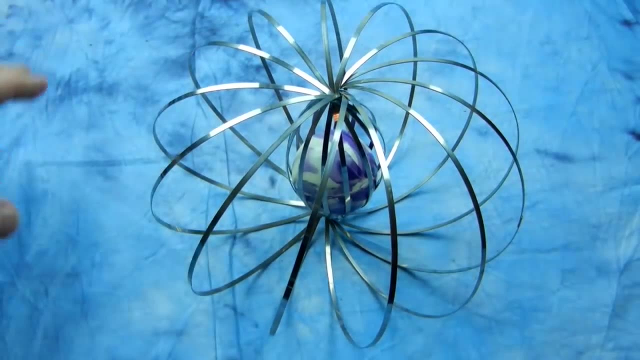 weren't stupid, by the way. But everything now is based upon Greek atomism. That's all. general relativity and quantum mechanics are is nothing other than atomism. If you don't know what atomism is, then I suggest you look it up. 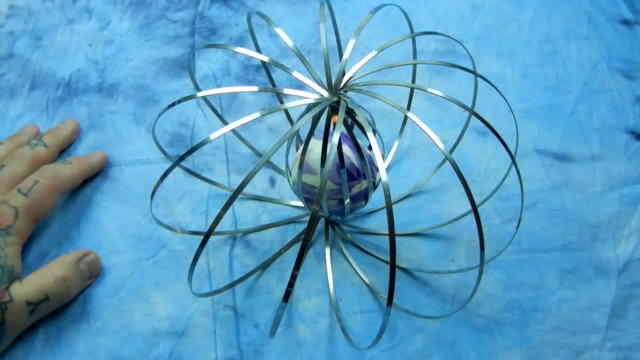 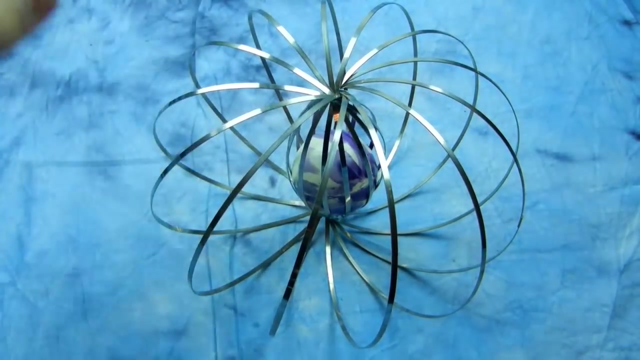 It basically means that the whole universe is just a giant bag of magical, unseen particles rolling around like BBs and volleyballs that are bumping into each other. Of course, they've never defined a field, Never, They never will define a field, because fields are particle free. We'll never define instantaneous action at a distance. 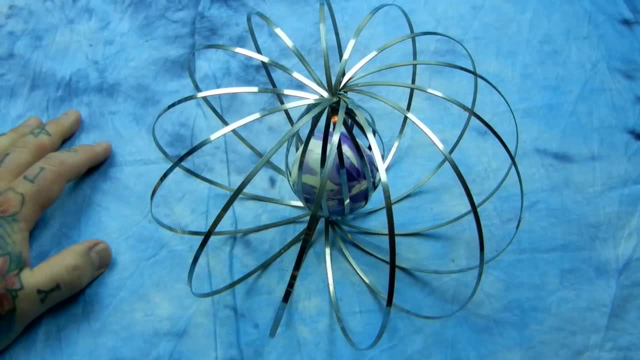 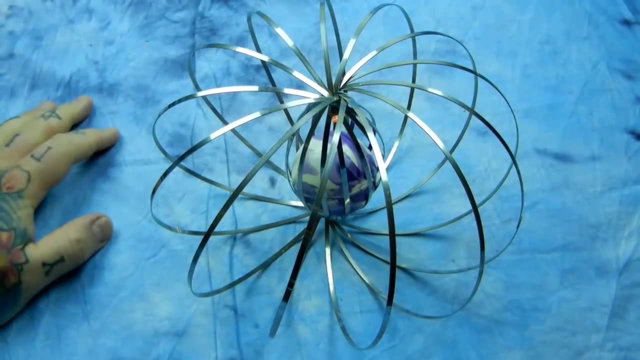 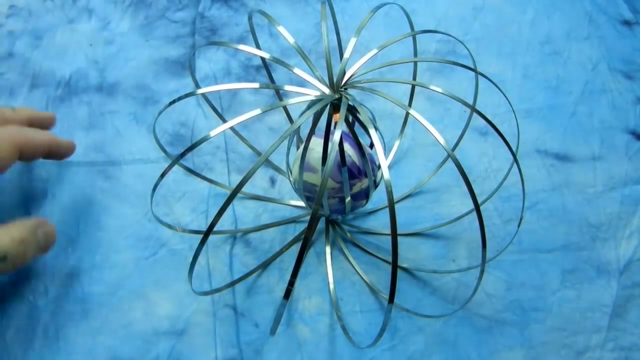 such as EPR. Look up EPR paradox. But we know that it exists. See faster than light, travel, instantaneous action at a distance contradicts the entire premise of general relativity and quantum mechanics, And so does the denotation of the term field, which has never been explained, never been defined. 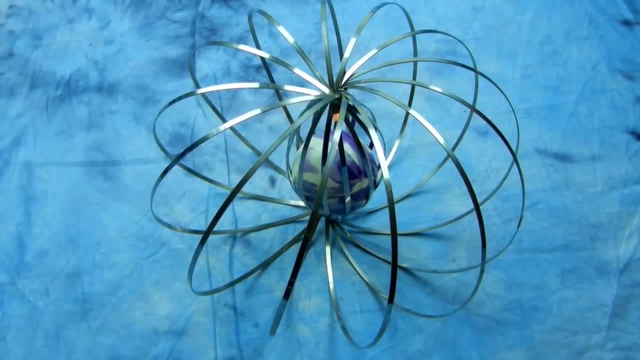 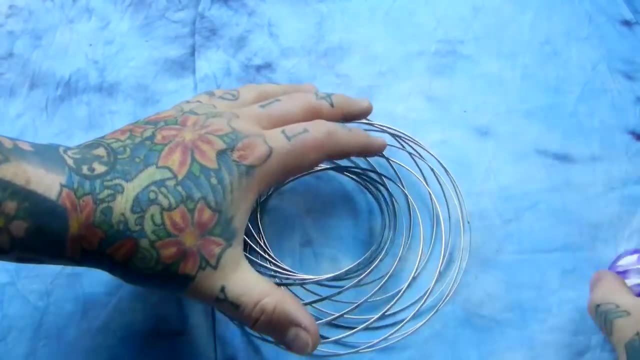 Human understanding is still in the stone ages. We think we're so advanced with our computers and our TV sets, but ultimately we're pretty stupid. So ultimately, let's look again, Remember back to the ferrocell. You see this again, This toroidal form that you see underneath the ferrocell, That's magnetism. 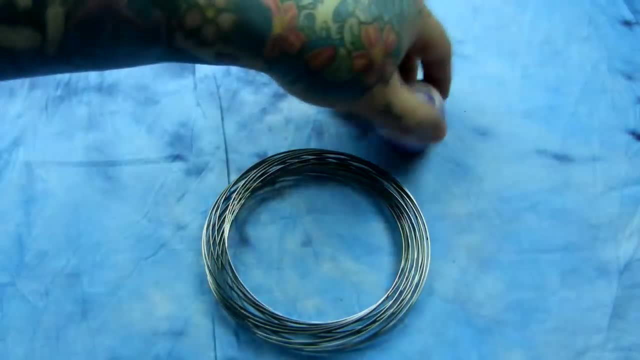 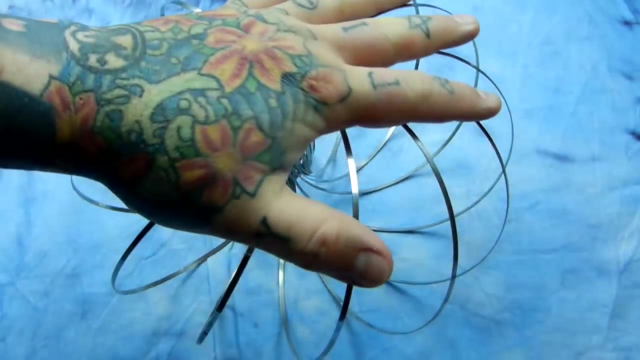 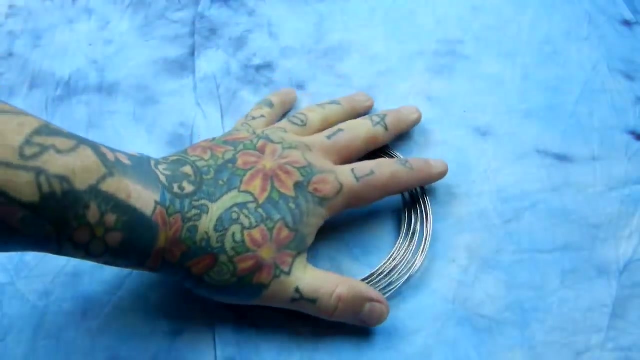 as painted by light, Tim Vanderely's wonderful invention. So you can think of this as a zero point ether pressure that has been released longitudinal. the expression of that form in transverse, reciprocating processional hyperboloid is magnetism. We have ultimately only one field. 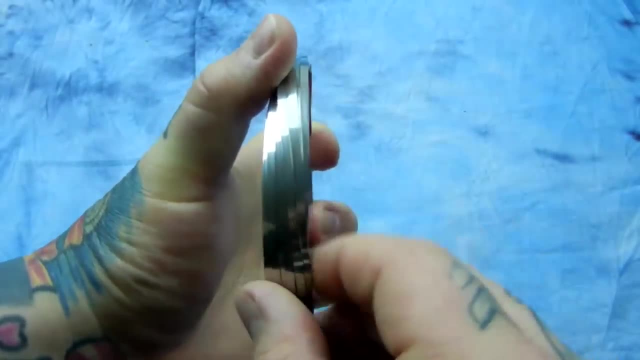 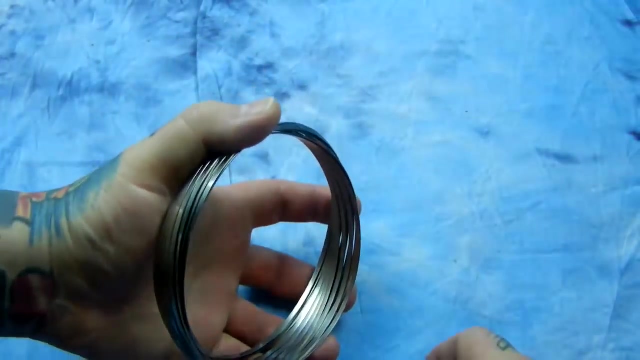 dielectricity, We have the loss of that field's potential, just like releasing charge on a battery, for example, And the release of that field- ie inertia, ie dielectricity- is force in motion. 100% of the visible. 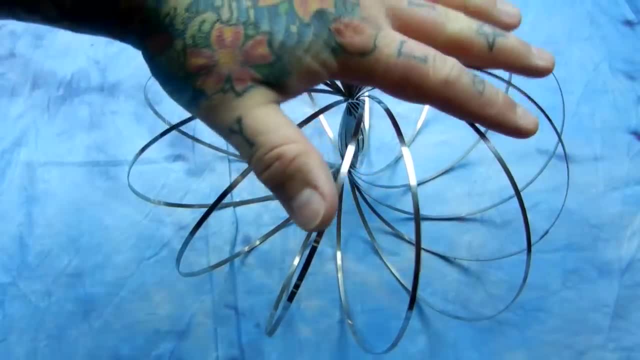 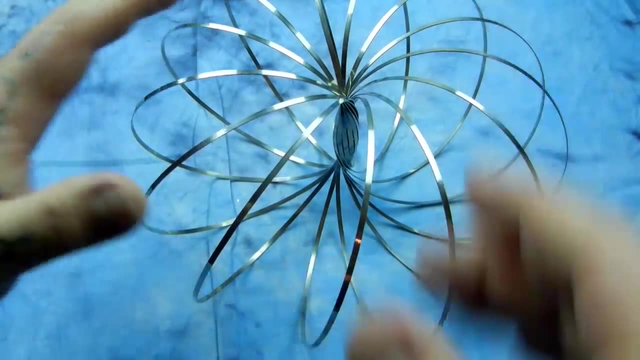 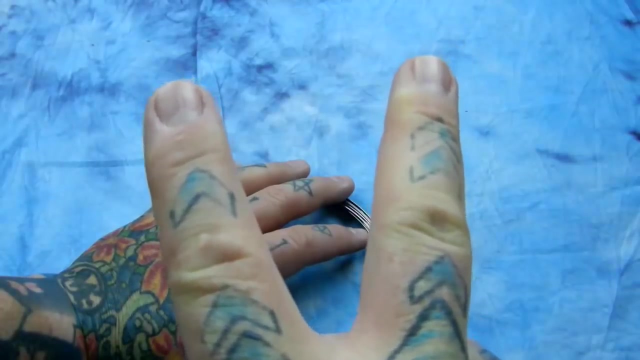 universe is. this Is magnetism. The entire atomic structure of an atom in picometers, as it measured in picometers, is due to magnetism, not dielectricity. So we have one field, one release of that field's potential, ie the 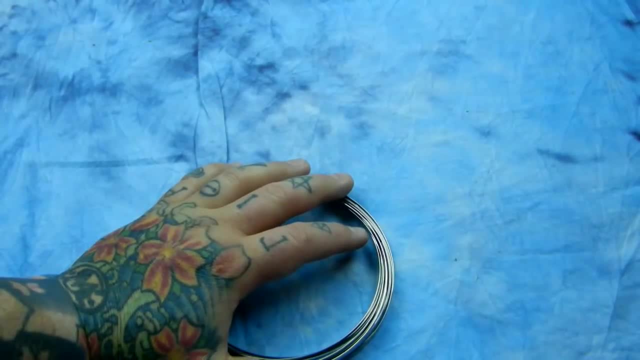 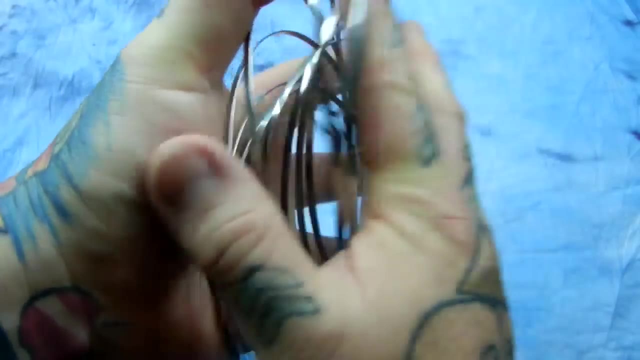 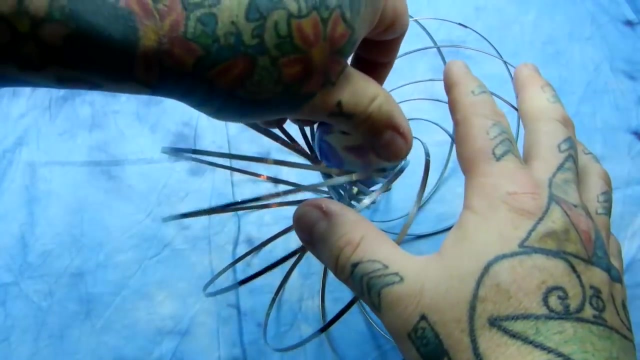 loss of that inertia as expressed in force and motion. And we have two field modalities, one being electricity, frequency and amplitude, and the other one being gravity, which is a dielectric condensate. We have a nucleus right here. we have tons. 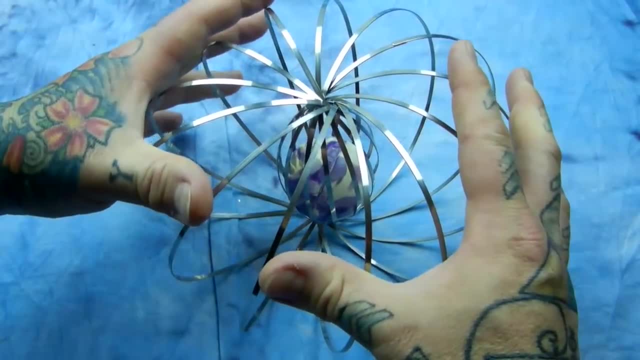 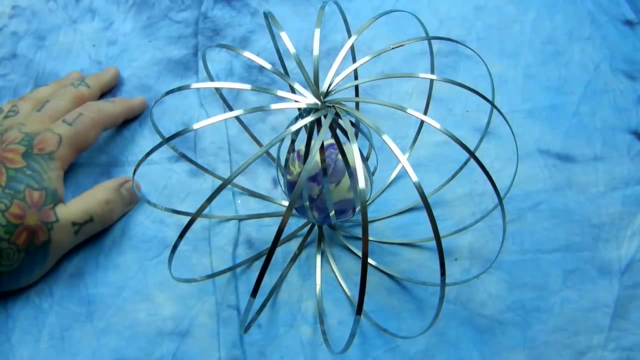 of magneto-dielectric space created. Space is not a thing. Space is neither a field nor a force. Space acts on nothing. Space does nothing. This is the ultimate brain virus and huge flaw that Tesla says over and over again, as well as others. 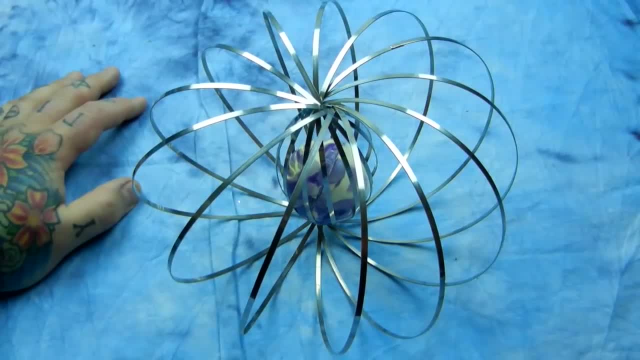 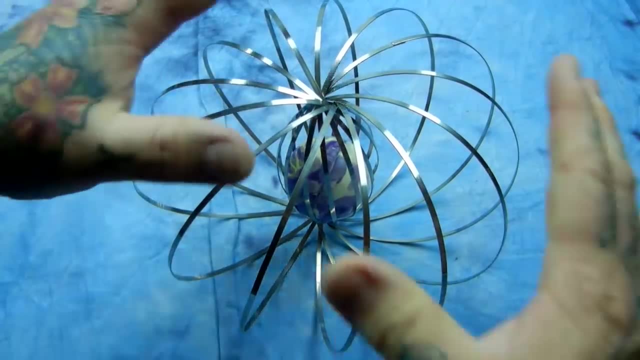 of general relativity is reified space as something that does something. It's like saying a shadow has done something. A shadow is the absence of something, The absence of inertia. let's just consider this central point here, which is not a point. 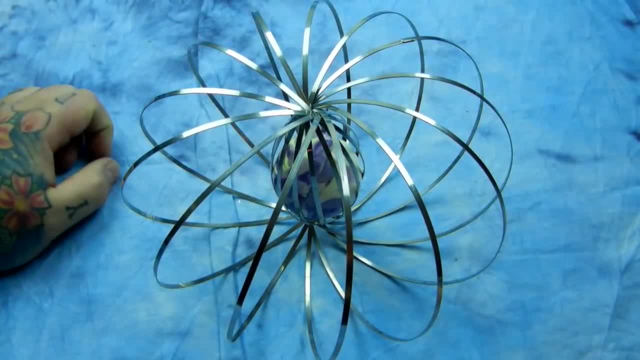 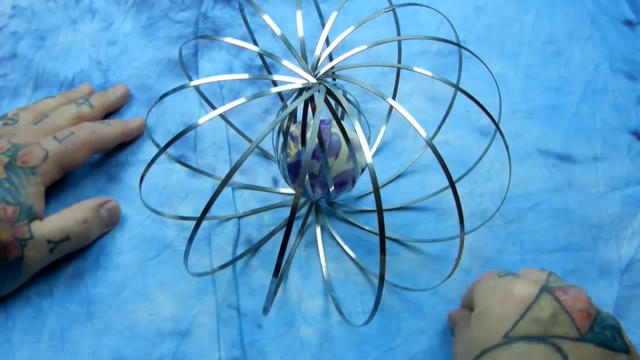 it's even prior to a point that the loss of that inertia is expressed in force and motion, leaves behind it a wake that us humans and our stupidity, all of us call space. We live in it, we breathe in it, because we're all existential. 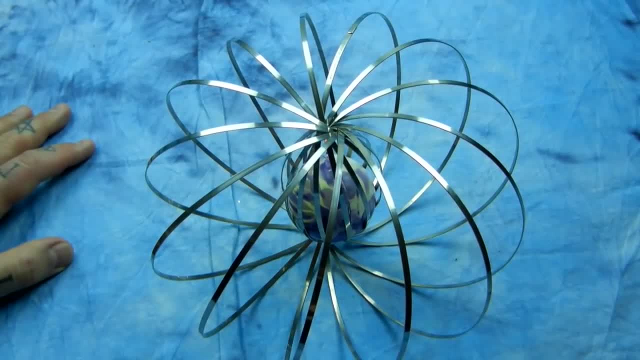 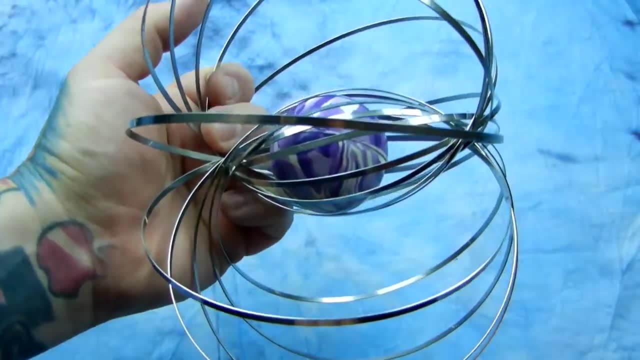 beings, but that space is neither a field nor a force. It does nothing and it acts on nothing. So here we have a dielectric condensate we call mass, or matter in its most simplex form- obviously An oversimplification, to be sure, with this model, which is a toroflux, by the way, 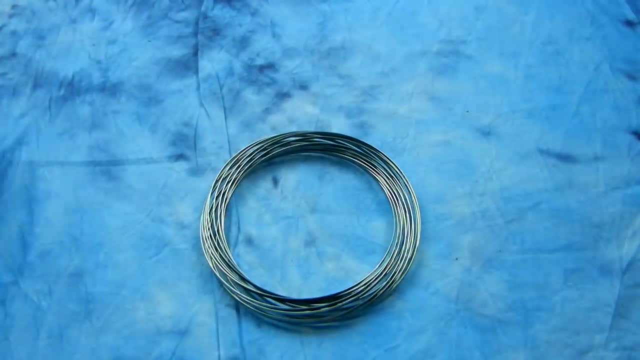 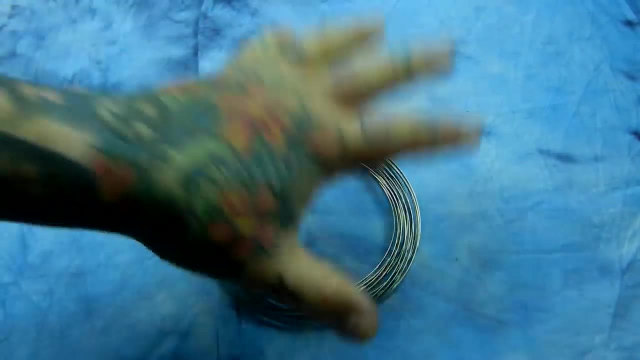 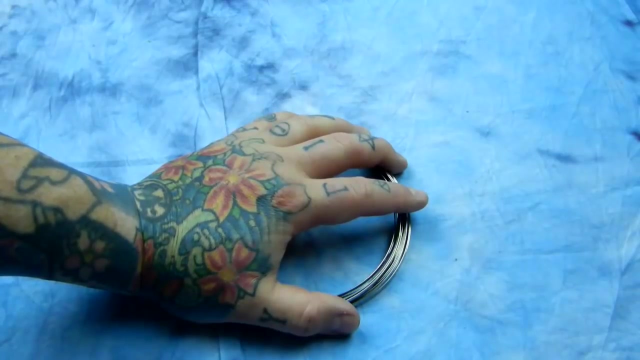 This cute little toy is called a toroflux. It's a neat little device that every little child should have that gets them thinking in multidimensional geometric fashions. So that's the irreducible simplicity of the universe. I have to stick fast to this and say that. 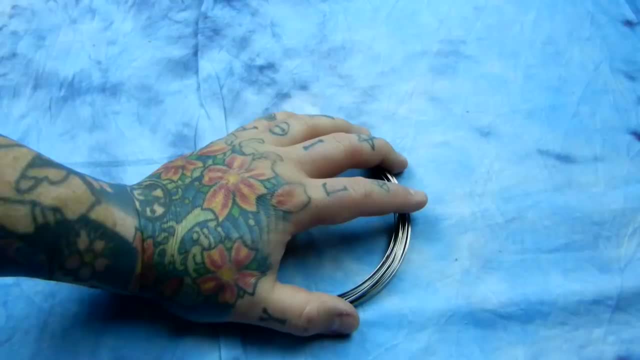 it's absolutely irrefutable As far as a grand unified theory it's already been discovered. whether anybody accepts it or not doesn't make any difference to me, I'm just happy to understand it. But we only have one field, that's dielectricity, ie the ether expressed longitudinally. That's the longitudinal. 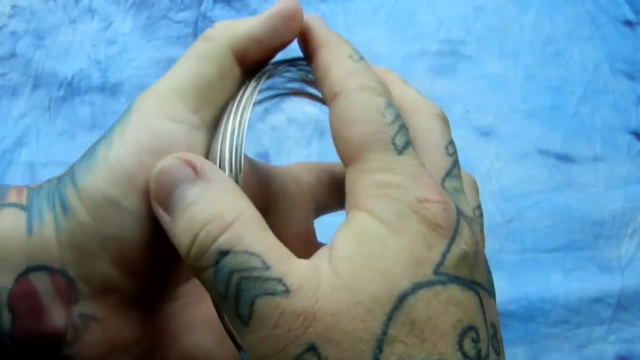 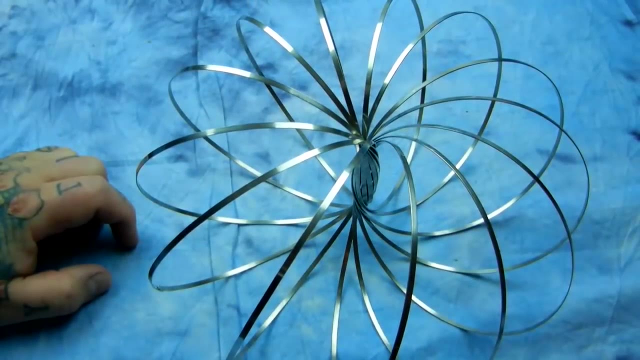 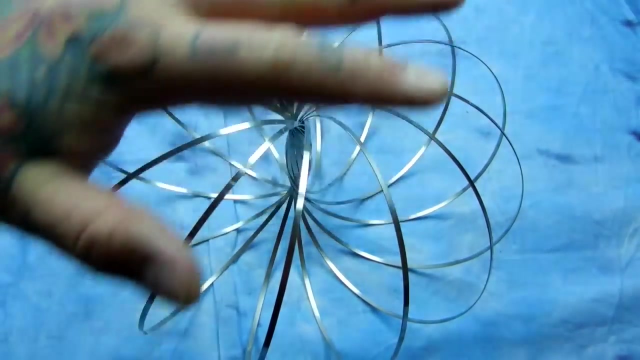 pulse found within transverse electromagnetism, We have the loss of that inertia, the loss of that acceleration as expressed by force and motion. Now, as I told you in prior videos, there's a huge difference, especially in field theory, between acceleration and motion. Increasing acceleration in terms of 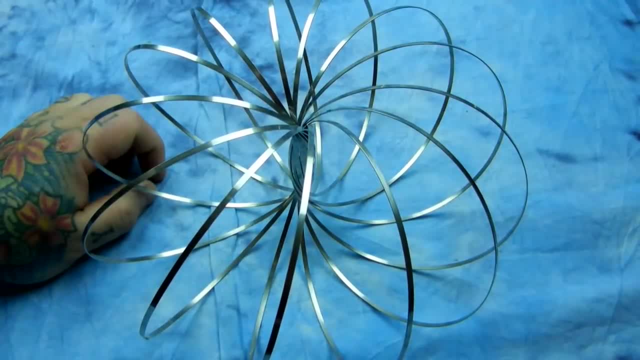 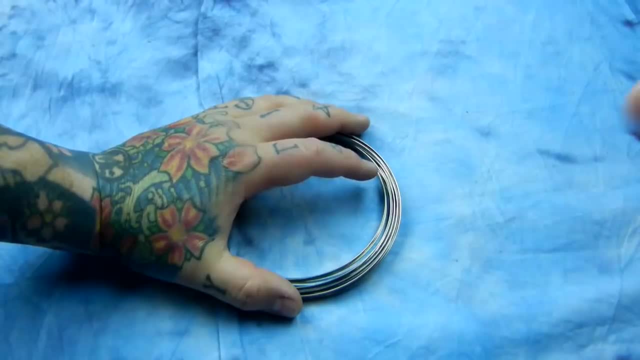 gravity, for example, which is an acceleration towards dielectric avoidance. Gravity is nothing other than dielectricity. Gravity is no different than turning on your TV set and actually shining a light off from the side and seeing little dust particles actually head to the TV set and stick to the TV set. 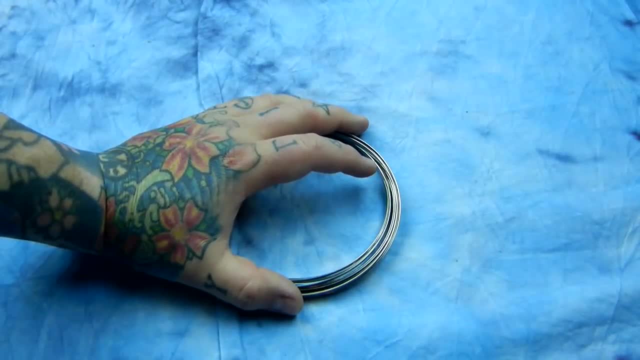 That's why your front of your TV set, especially little CRT tubes, got so dusty. The dust in the air would go gravitate to the front of the TV set. That is the exact same thing as gravity. People think that that is an electrostatic. 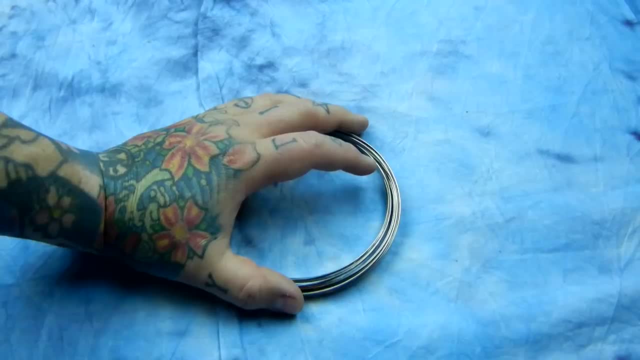 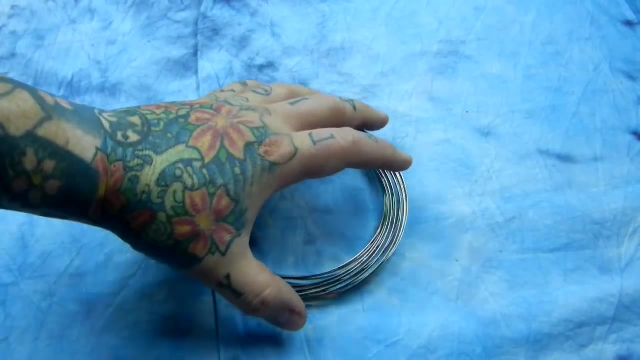 charge, or like you charge a balloon up and you pull someone's hair to it. That same acceleration- not force, that same acceleration is what we ignorantly call gravity. Gravity itself is an autonomous acceleration, of which a lot of people call it, incorrectly, a force. 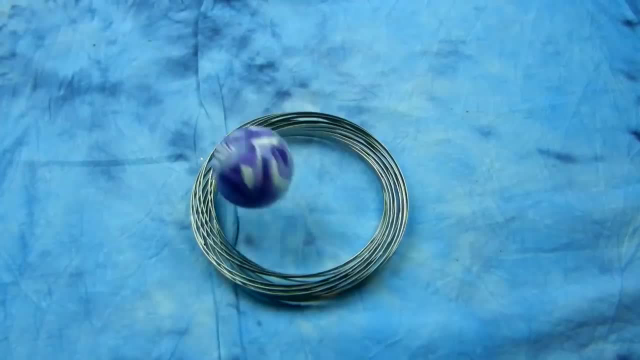 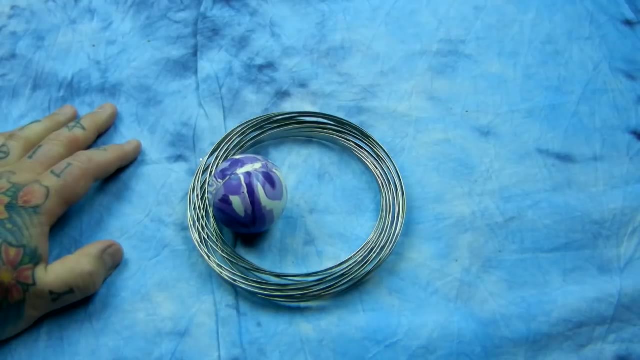 does not exist. It's like: what do you mean? gravity doesn't exist. Obviously, I can drop this and there's gravity. What I mean specifically is that gravity does not exist. It is not an autonomous force, It's definitely not a force. 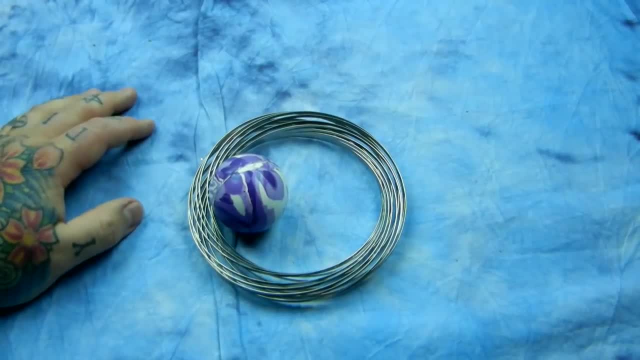 Which, of course, even the idiots of general relativity and quantum mechanics will admit to. They call it an acceleration: Acceleration of what By what. We need explanations, not descriptions, And all that general relativity and quantum mechanics provides are descriptions not. 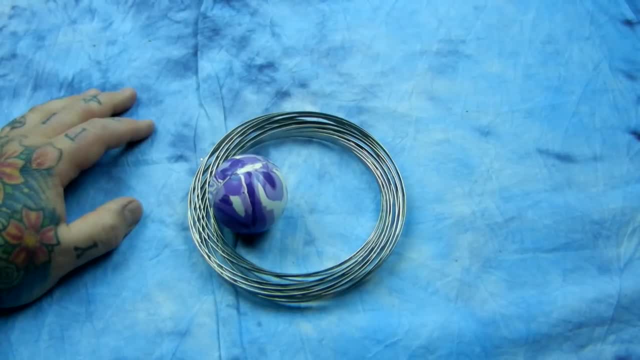 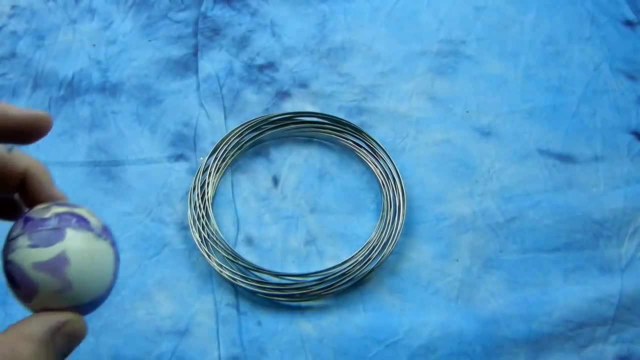 explanations. It is dielectric acceleration, It's dielectric avoidance. Okay, It is the loss of force in motion, Because there are no straight lines in the universe. What we think are straight lines in the universe are infinitely slightly curved. There are no. 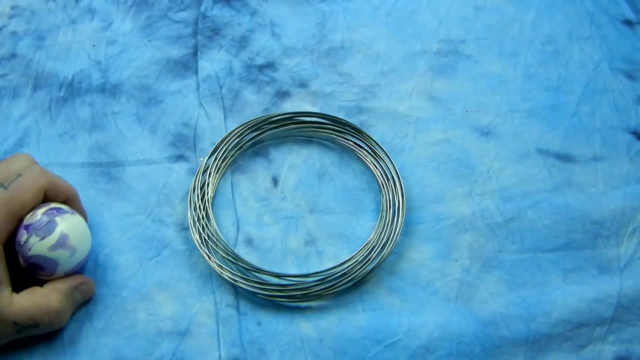 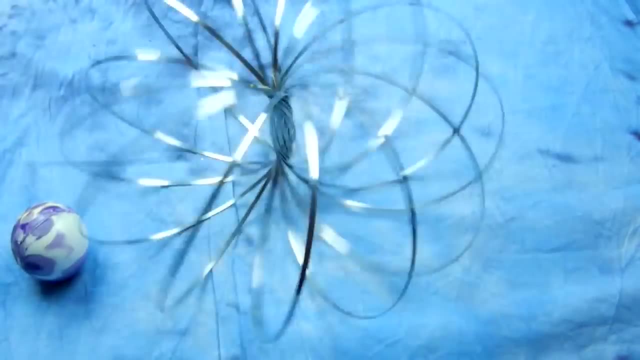 there's not a single straight line anywhere in the universe. None, nowhere, ever, never Doesn't exist. So hope I made that very simple. We have one field, We have the loss of that field expressed as force in motion, And we have two field modalities: One expressed as a dielectric, 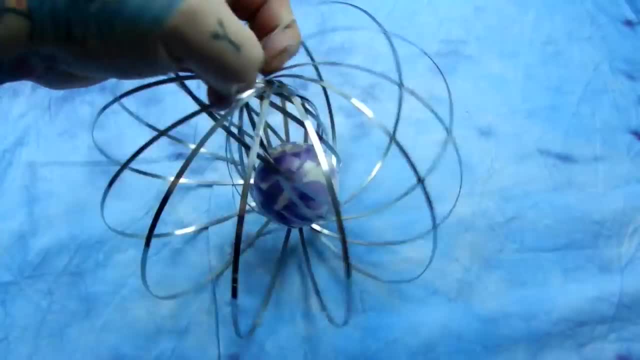 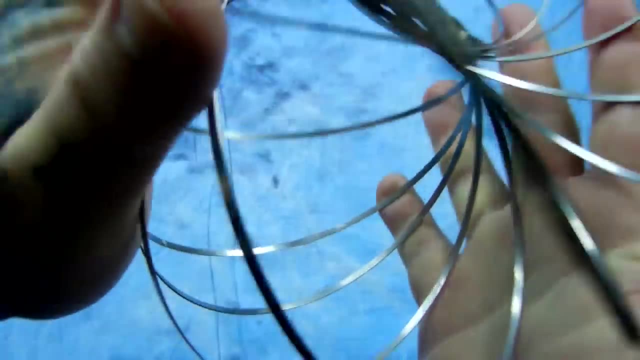 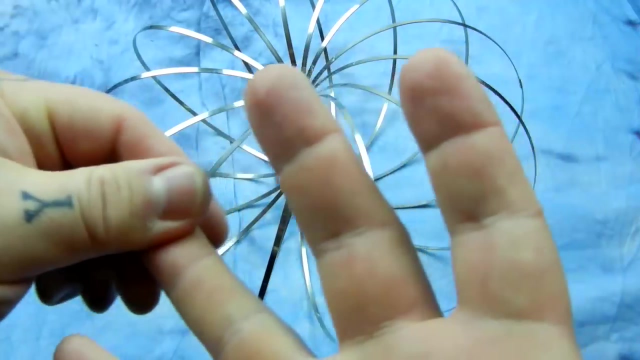 condensate, which we call matter mass, Okay, And the other one which is expressed by longitudinal transverse force and motion, Transverse electromagnetism, expressed in frequency and amplitude, what we call electricity. So dielectricity, electrostatics, electricity, magnetism and, quote unquote, gravity. 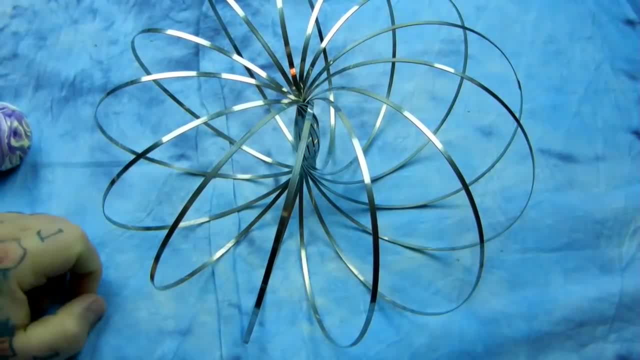 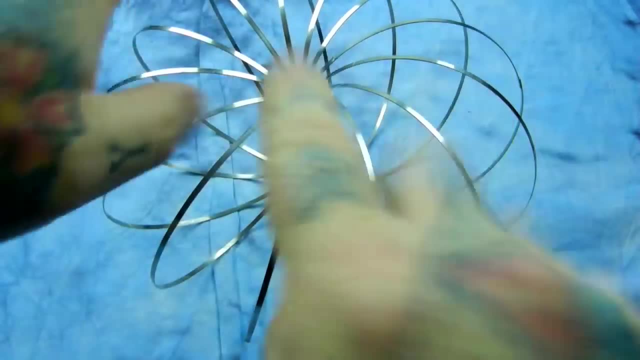 are one thing only. It's our only pathetic human understanding of the nature of the universe that we think these are four separate things. Really, they're just one thing. They're a hydra, A single beast with four heads, if you want to talk about it that way.